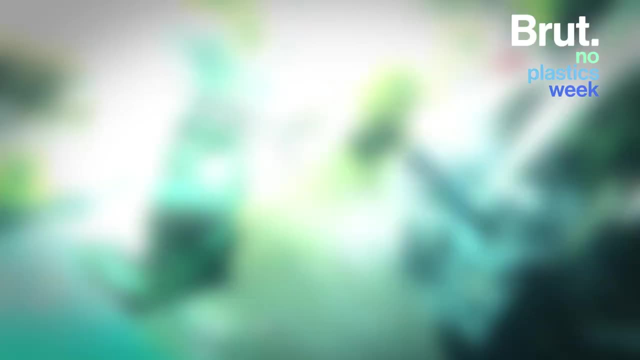 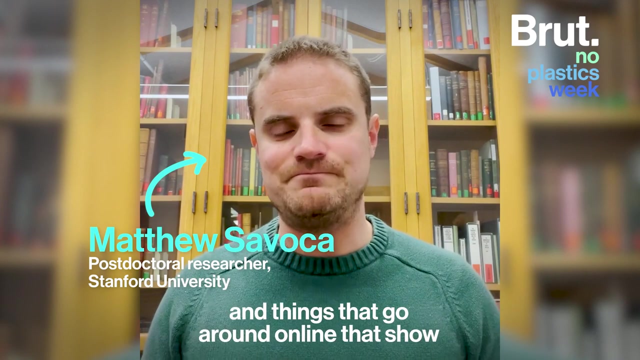 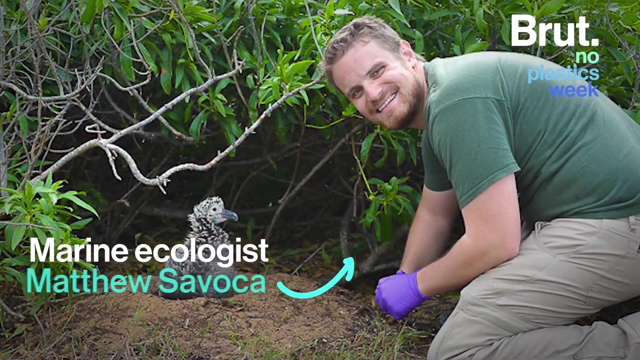 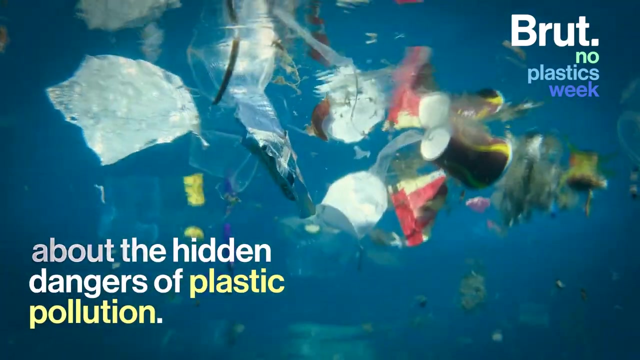 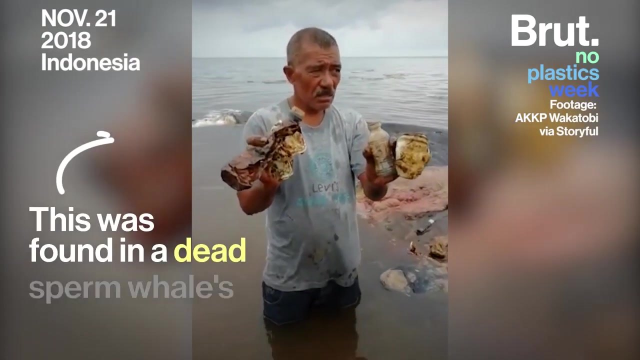 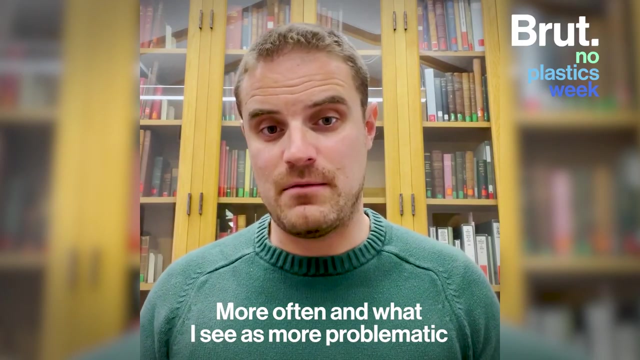 You'll see all these different images and videos and things that go around online that show really dramatically how plastic can kill animals at sea. It can rip through their intestines or it can fill them up or block the passage of food through their bodies More often, and what I see as more problematic is the extent at which plastic and 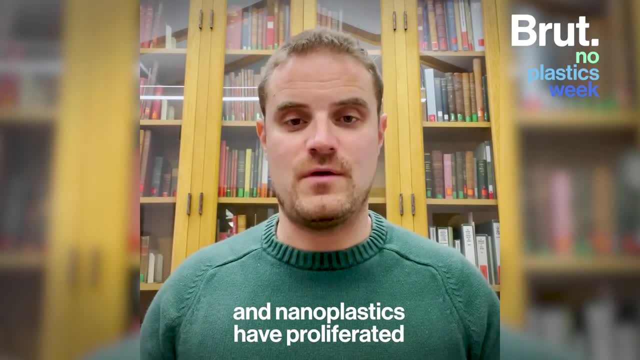 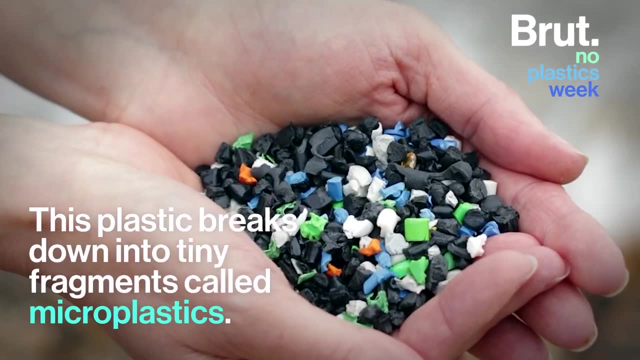 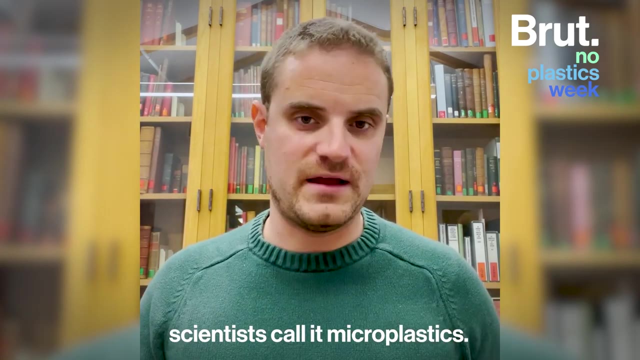 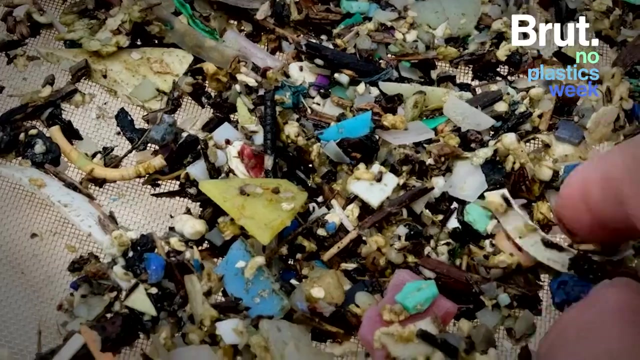 these little microplastics and nanoplastics have proliferated through the food web. When plastic gets smaller than five millimeters, scientists call it microplastics, And these plastics are very harmful because they can be easily ingested by a huge number of marine species. They're also very hard to clean up. How do you clean up a tiny, tiny, tiny? 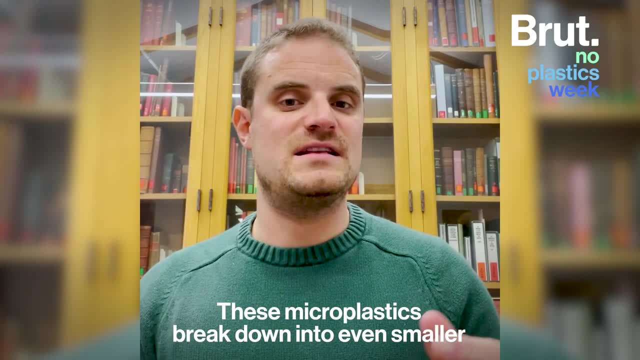 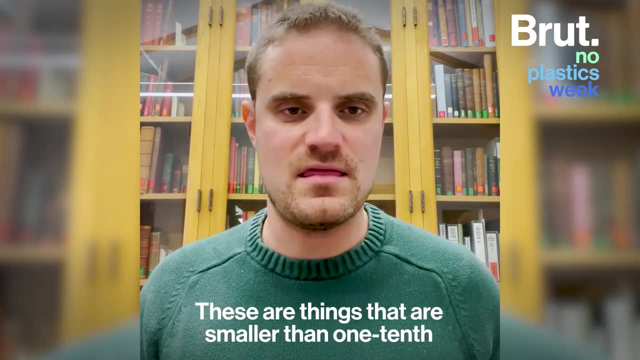 bit of plastic Really really hard. These microplastics break down into even smaller pieces of plastic, called nanoplastics, that are so small. These are things that are smaller than one-tenth of one millimeter And when plastics get that small they can pass through your gut wall and 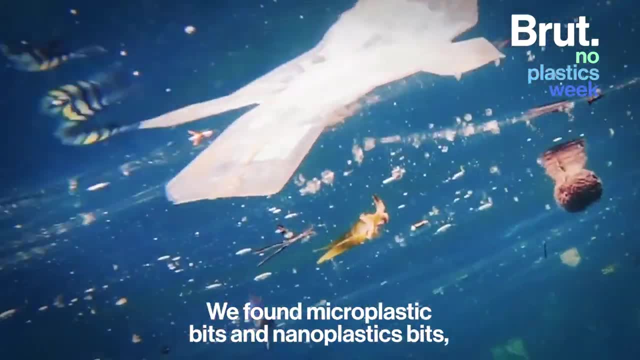 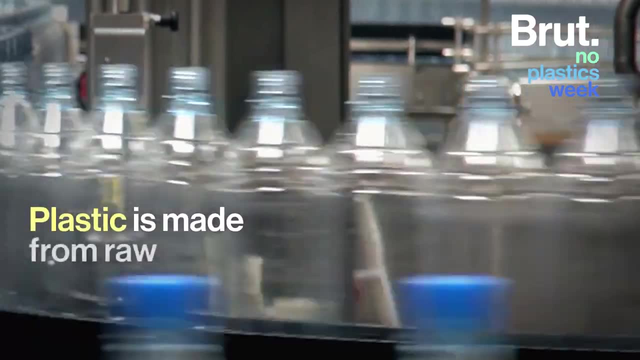 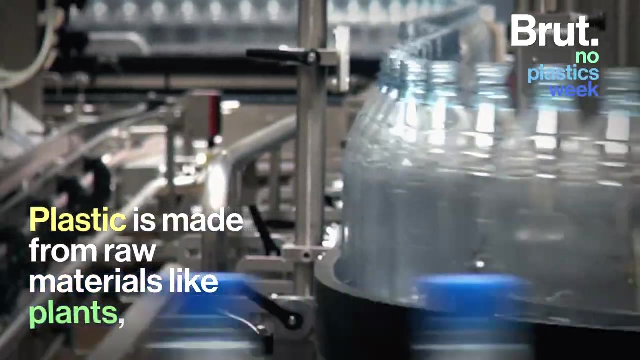 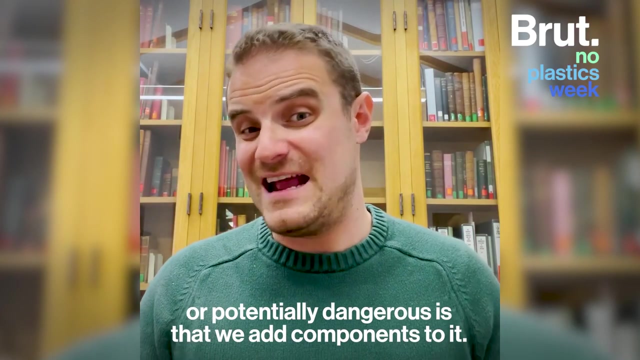 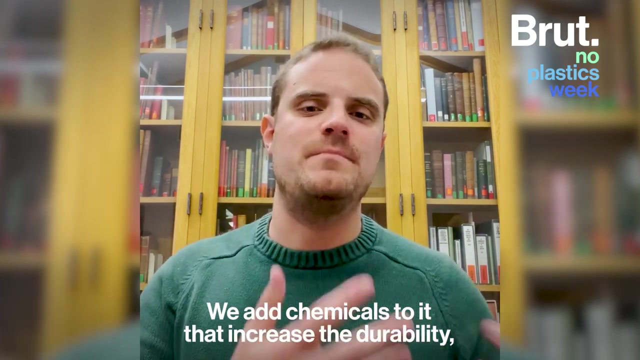 into your body tissues. We find microplastic bits and nanoplastic bits, more importantly in things like livers and muscle tissues and gills of fish. What makes plastic particularly dangerous or potentially dangerous is that we add components to it. We add chemicals to it that increase the durability. 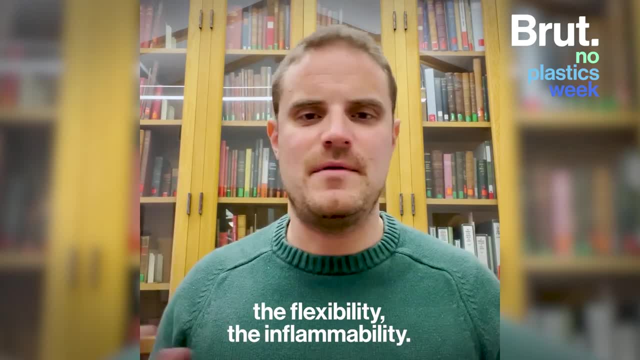 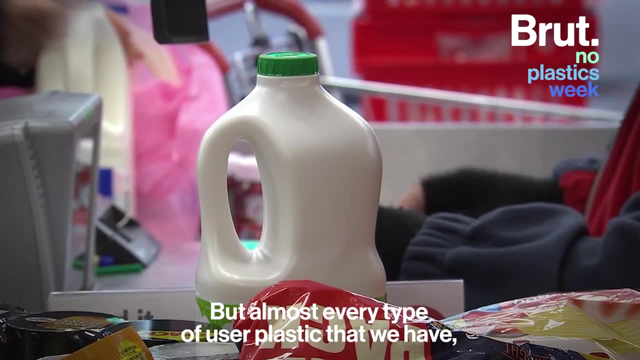 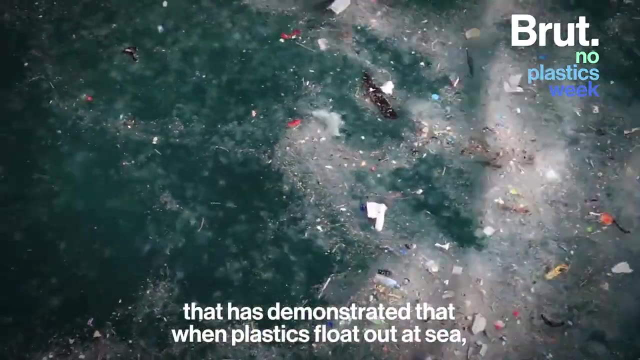 the flexibility, the inflammability. These are much more worrisome than the plastic backbone itself. But almost every type of user plastic that we have have these additives. But also there's been a lot of good research that has demonstrated that when plastics float out at sea they actually act. 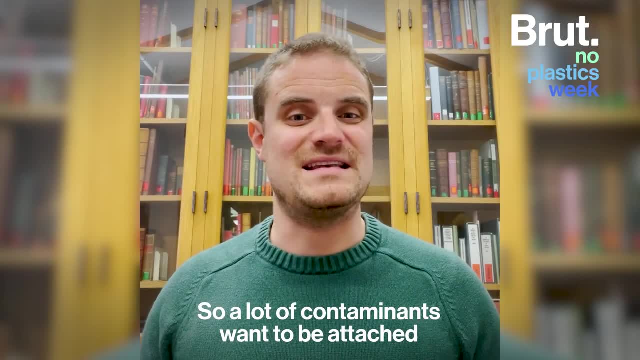 as a contaminant sponge. So a lot of contaminants want to be attached to something hard, And plastic is a great substrate for which these additives can be used. So plastic is a great substrate for which these additives can be used. So plastic is a great substrate for which these additives can be used. So 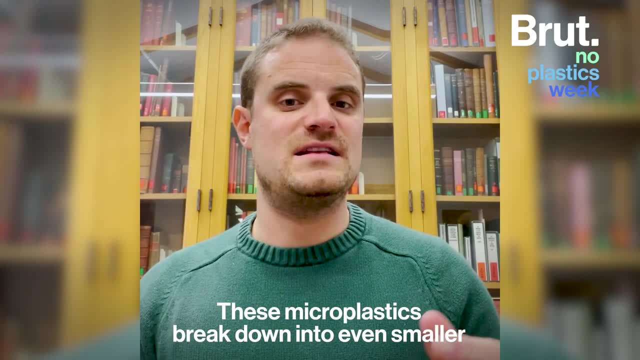 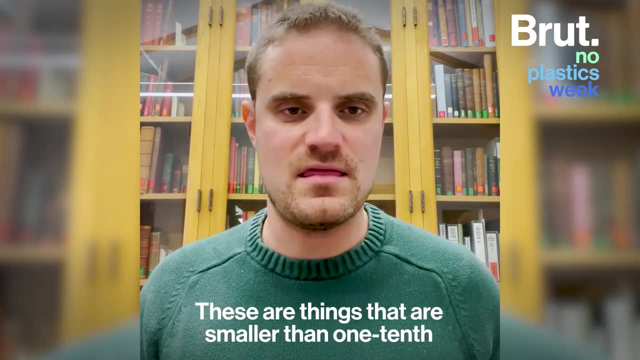 bit of plastic Really really hard. These microplastics break down into even smaller pieces of plastic, called nanoplastics, that are so small. These are things that are smaller than one-tenth of one millimeter And when plastics get that small they can pass through your gut wall and 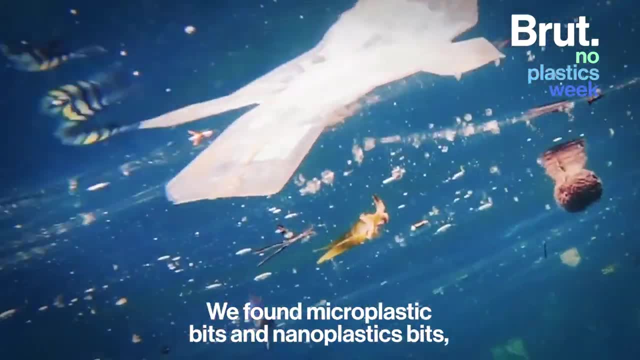 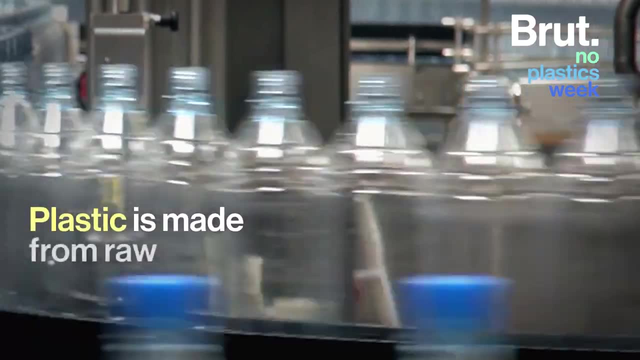 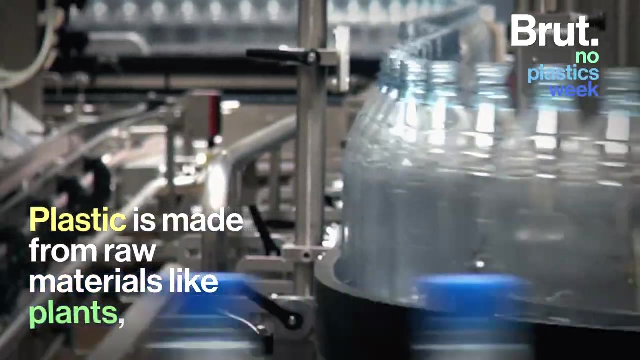 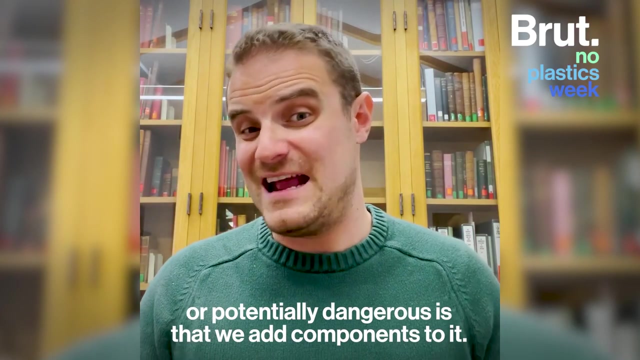 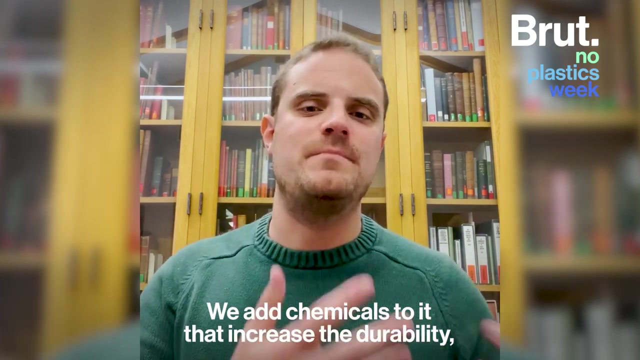 into your body tissues. We find microplastic bits and nanoplastic bits, more importantly in things like livers and muscle tissues and gills of fish. What makes plastic particularly dangerous or potentially dangerous is that we add components to it. We add chemicals to it that increase the durability. 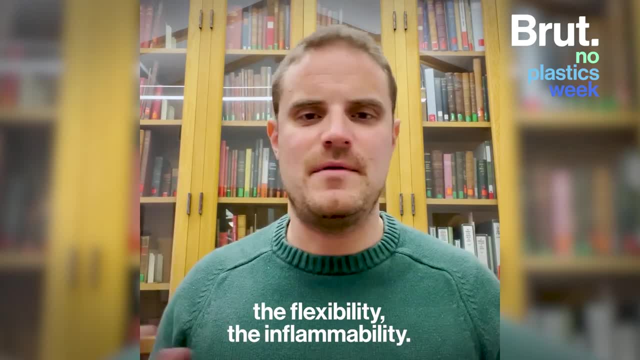 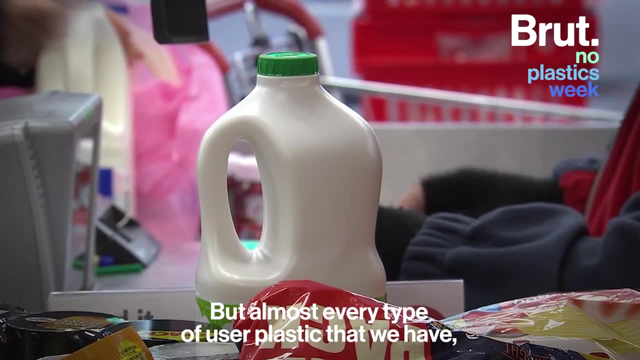 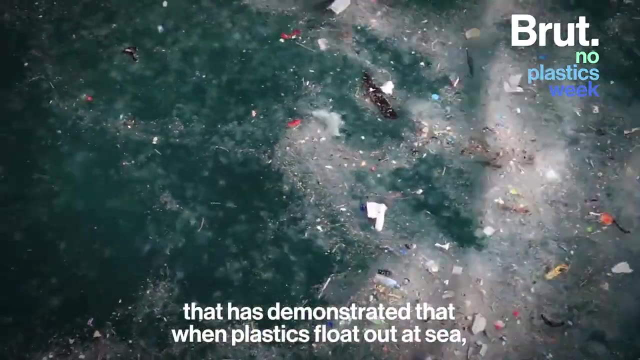 the flexibility, the inflammability. These are much more worrisome than the plastic backbone itself. But almost every type of user plastic that we have have these additives. But also there's been a lot of good research that has demonstrated that when plastics float out at sea they actually act. 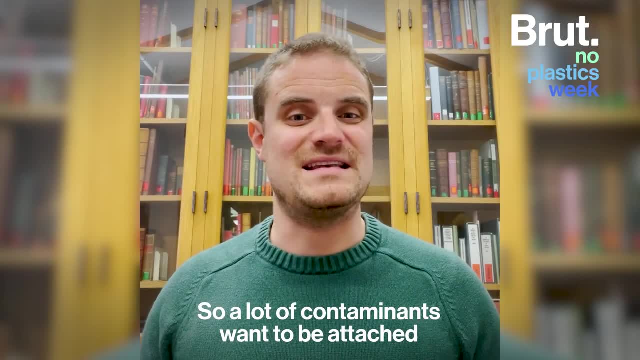 as a contaminant sponge. So a lot of contaminants want to be attached to something hard, And plastic is a great substrate for which these additives can be used. So plastic is a great substrate for which these additives can be used. So plastic is a great substrate for which these additives can be used. So 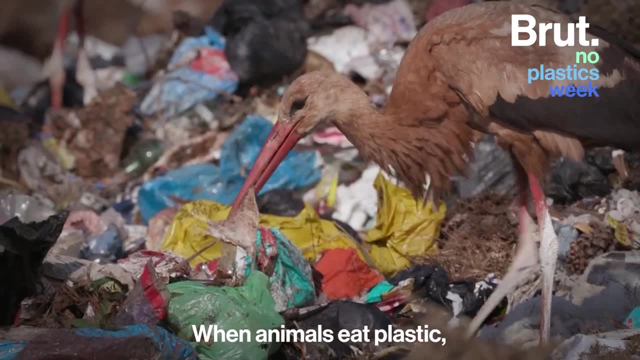 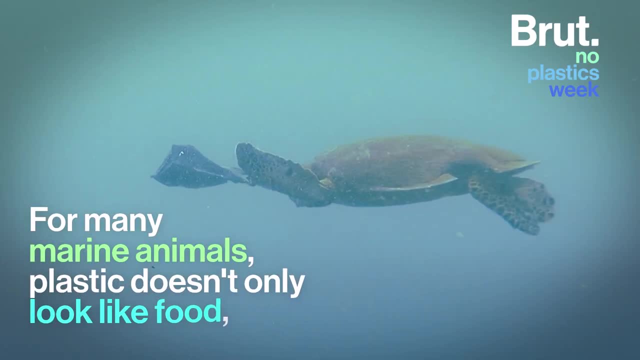 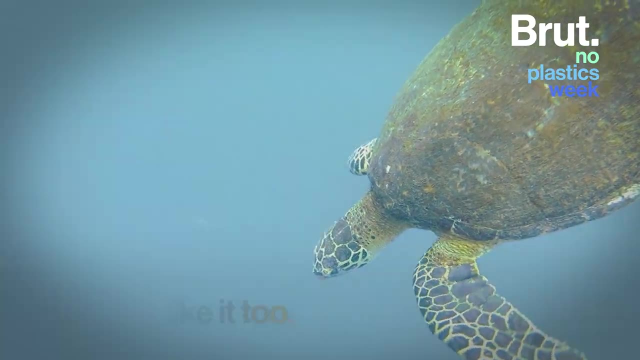 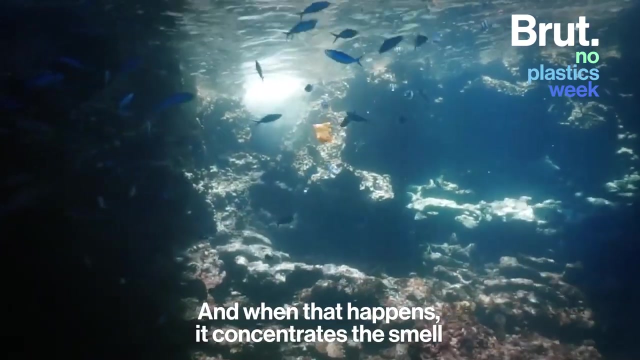 these contaminants can associate with. When animals eat plastic, they can get this dose of contaminants that can be potentially detrimental for their system. Plastic attracts a lot of marine life In addition to these contaminants, things like algaes and phytoplanktons, And when that happens, 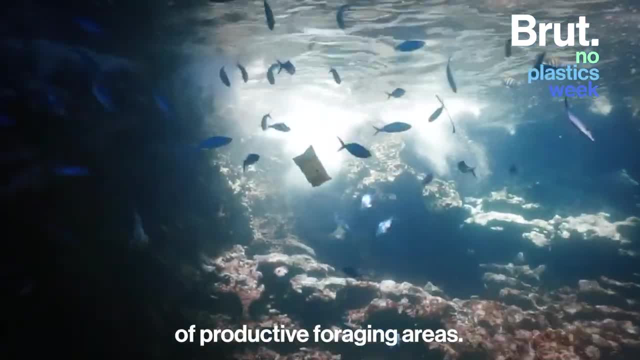 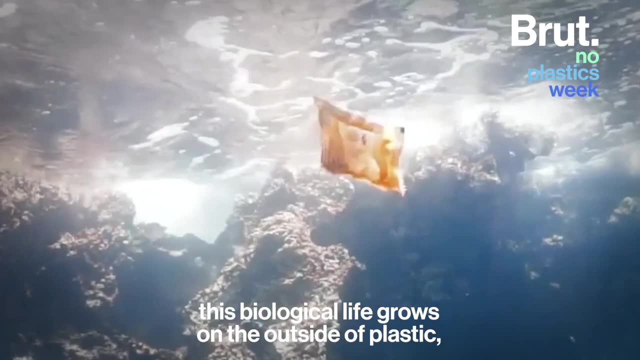 it concentrates the smell of productive foraging areas, And so what we've found is that plastic can found, and shown in a number of different experiments now, is that when this biological life grows on the outside of plastic, it makes plastic seem superficially attractive to these. 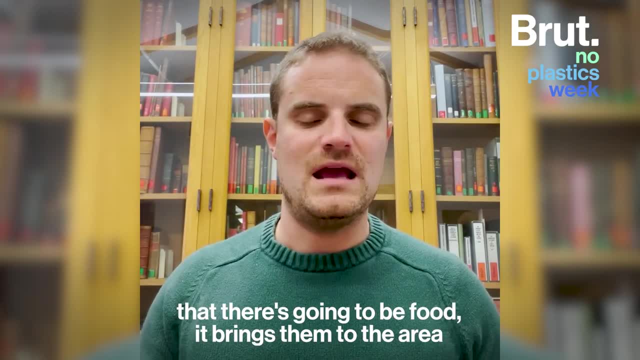 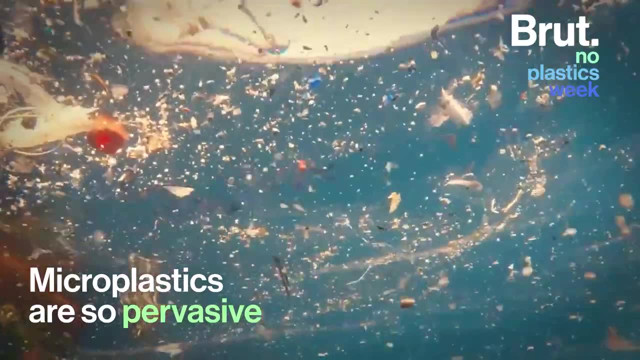 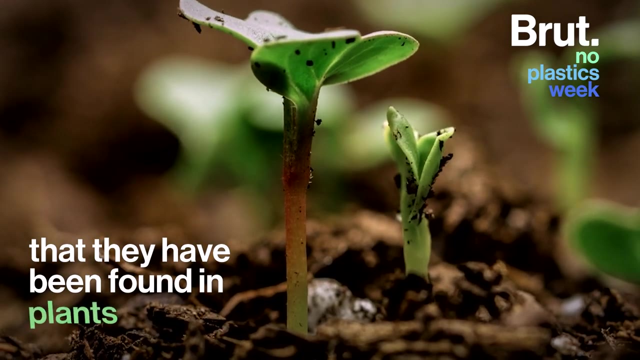 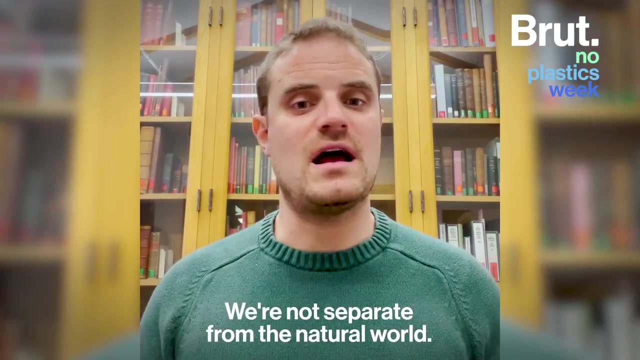 animals, And once their nose tells them that there's going to be food, it brings them to the area where there might be plastic debris, perhaps instead of food or in addition to food. So we're not separate from the natural world Anything that we can find out about these fish.